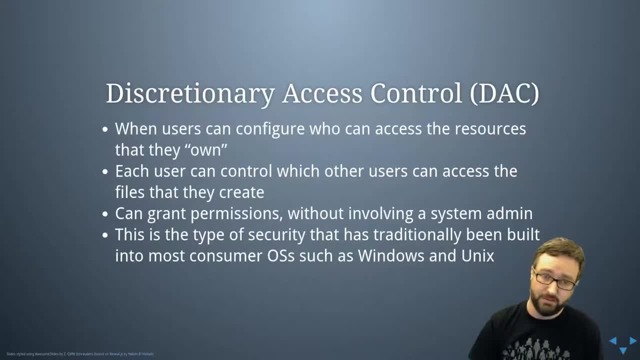 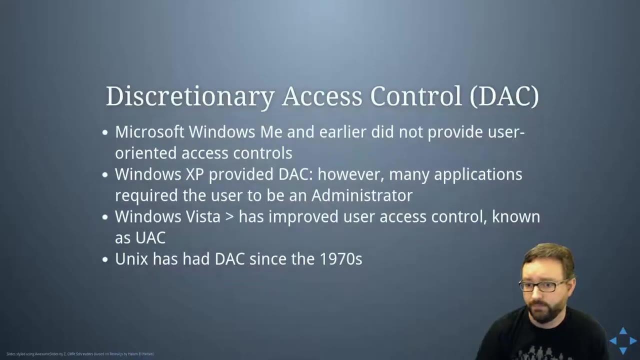 like consumer operating systems. So if you're using a Linux or Mac or you know Windows system, then it's based on discretionary access control. So you get to create a file and if you've got multiple users on that system you get to say who gets to access those files. If 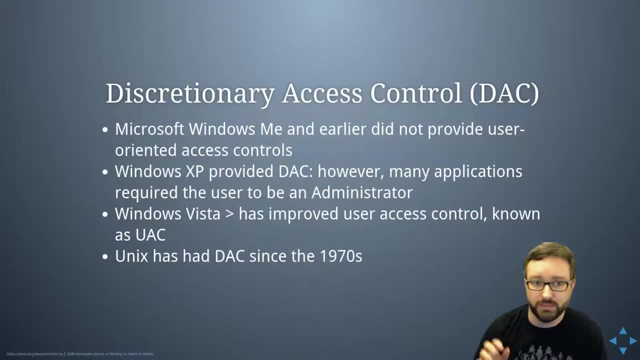 you look at older versions of Windows, so Windows Millennium Edition- if you've got the misfortune to have experienced that firsthand- and anything earlier like Windows 95 and so on, They didn't actually provide any user-oriented access controls at all. So basically, as soon as you look, everyone's 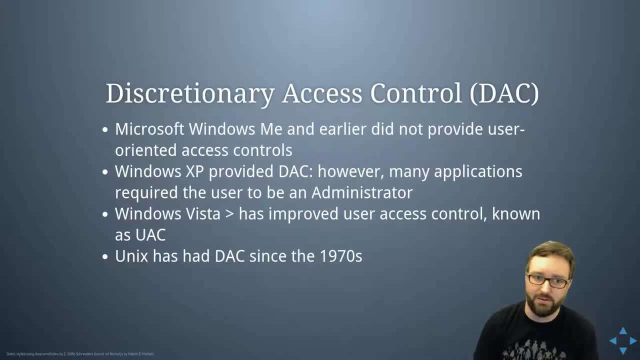 an admin there. well, there was nothing other than the ability to do everything. but when you log in, that login screen is literally like if you know the password, you get to have your desktop wallpaper and those set of icons, But you know there's nothing else there. And then it was in Windows XP where they actually 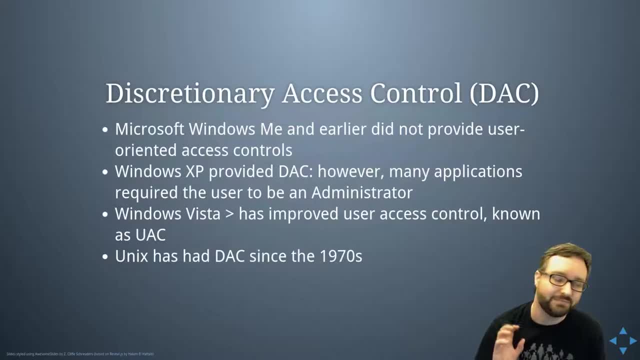 started to introduce discretionary access controls but because of the history that Windows had of everyone running as administrator- like a lot of software that existed for Windows which they wanted to be backwards compatible for wouldn't work unless you were an administrator and so you kind of perpetuated this idea that you had to be an admin on on Windows XP. 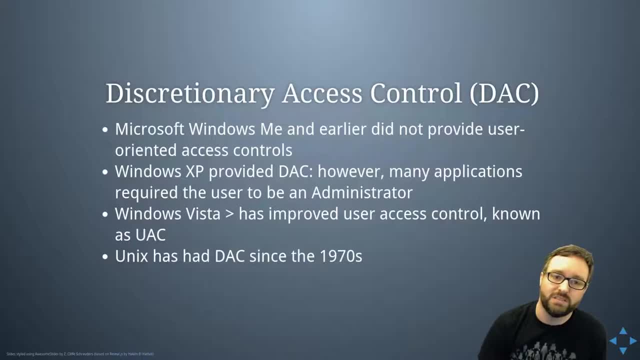 and when Windows Vista came along, they tried to ease that transition of like, allowing you to have the ability to escalate to admin when you needed it. and they introduced UAC, which is basically those pop-ups. it's like trying to install some software. Are you sure you've got the right software? 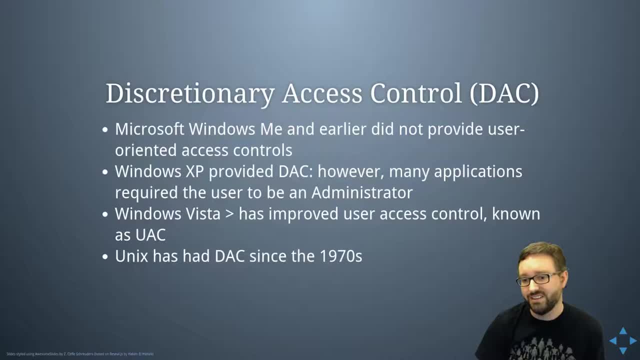 You want it to be able to do this. you know it's trying to do some kind of admin action, which is a great idea in terms of like it's much better than everyone running as an administrator all the time. but it got panned for the usability. 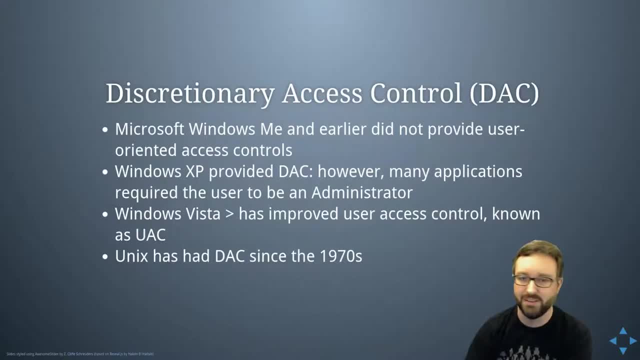 because suddenly security was in everyone's face. like: why am I being prompted for this? like, of course I want to allow it, do I clicked it and so since then they've tried to improve the UI experience of that, but it was actually a step forward in terms of security being better than the. 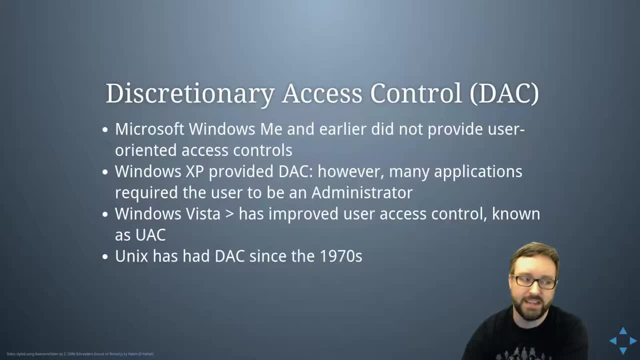 what it was before then, and they've. they needed to tweak the kind of actions that prompted the dialogue and the rest of it. but meanwhile Unix, including the earliest versions of Linux, have had discretionary access control since the start, so since the 1970s, or you know, when it was first released- has has. 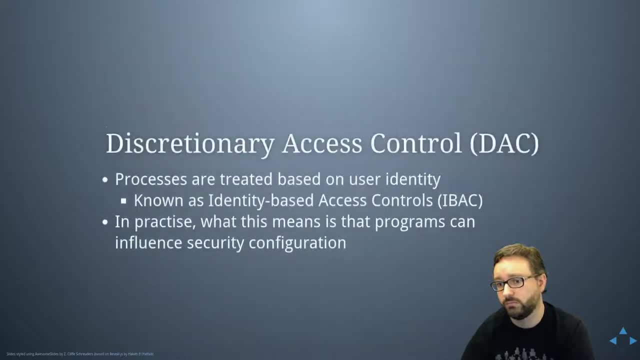 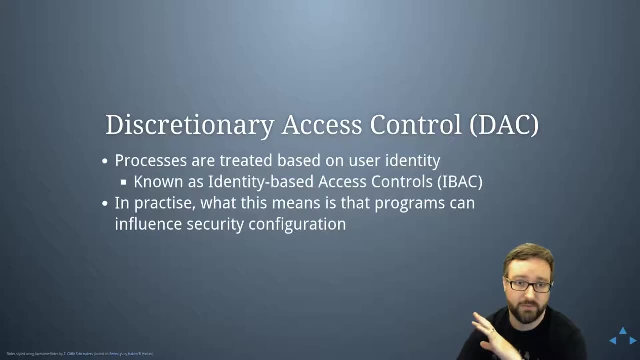 always had that built into the system. so what you happens normally on a discretionary access control system, like where you you know, like Linux for example, you start a process up. so if I'm a user, I'm sitting at the computer on a start program, the process starts and it is has. 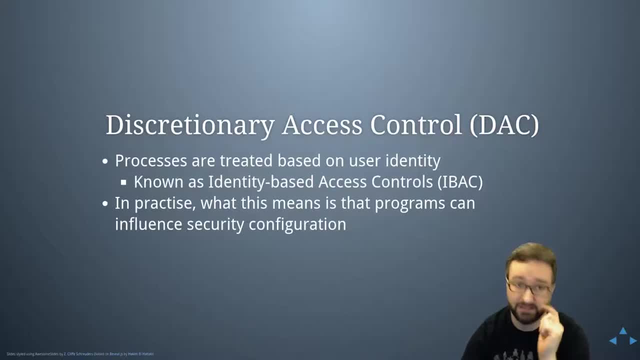 the user identity associated with that process, so the UID, and and then all the decisions that get made are based on that UID. so when you have a system where all the decisions are basically based on the identity of the person, that's also known as an identity based access controls. 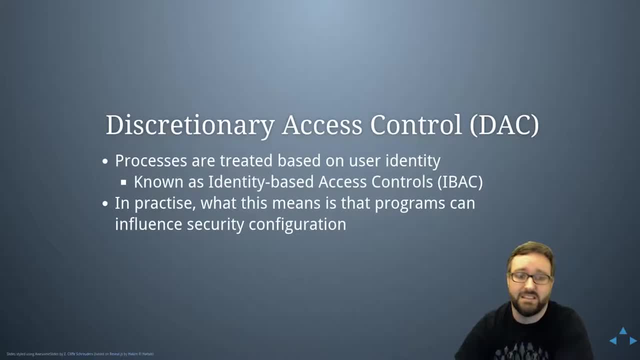 so in practice, what that means is all the programs are running around with all of your privileges, and so there's a bunch of like. there's a problem of ambient authority, so you've got a lot of processors that have a lot of power to do things in your name. that's how these systems are designed, basically, but so 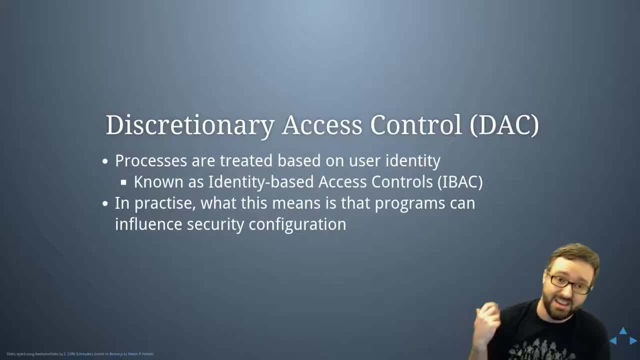 hypothetically- not that hypothetically actually- a program running can just like set all the permissions on all of your files quite easily, can do all the things to you on the system and you're kind of working on the assumption that they're working for you. but that's. that is the the way that most operating systems work as a starting point. 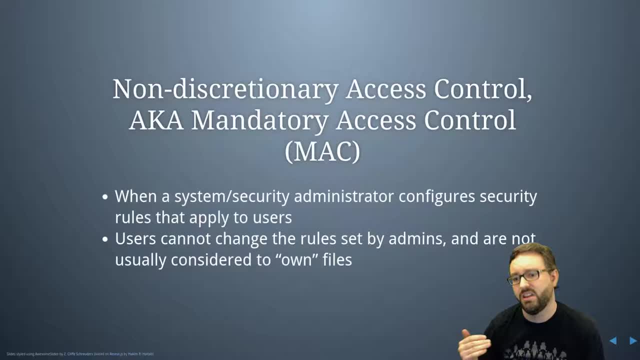 so non-discretionary or mandatory access controls is where the policy is defined by someone else, like an administrator, so it's defined for the system and then that applies to all the users. so users don't get to choose, they don't get to set the rules. admin sets the rules and 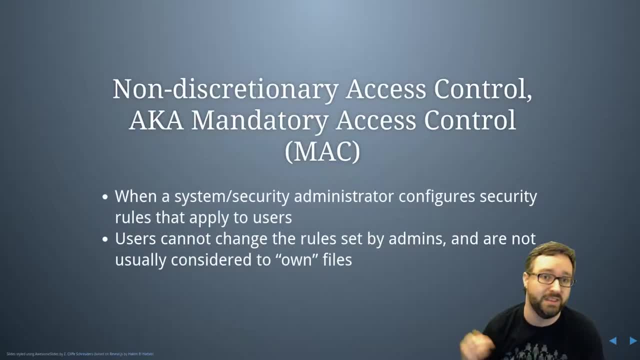 if you create a file, well, you, just you happen. you might happen to be the creator of that file. that doesn't really give you the ability to set the rules for that file. that's the job of the system administrator. so the reason why we say this non-discretionary or mandatory is that traditionally, 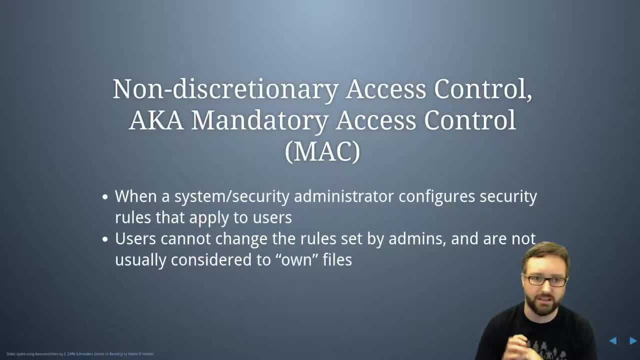 mandatory access controls were defined based on like a formal notation, basically like this lattice structure of mathematical set of rules. it's a set of rules about who's allowed to access what um and it's an active area of, of research. but more broadly, the term non-discretionary and also the term mandatory access controls gets used. 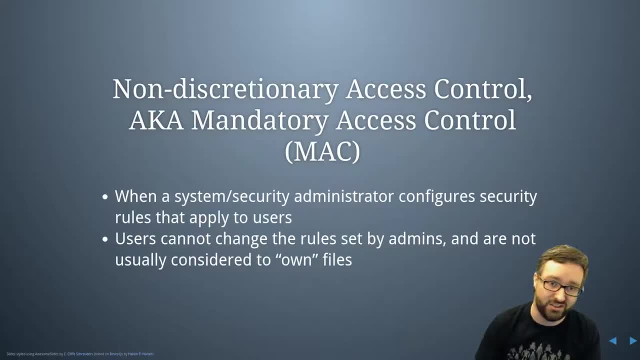 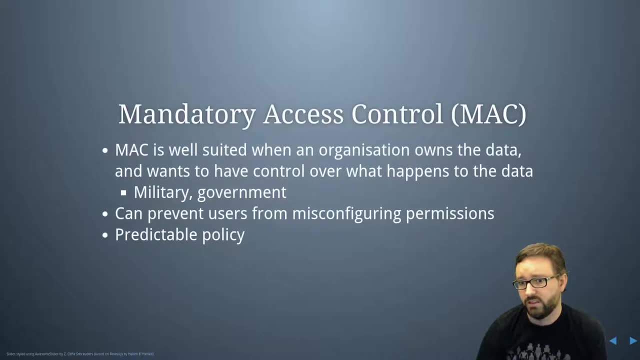 in the broad sense of being that the users don't get to choose um. so you know you might come across either of those terminologies, so so yeah, so mandatory access control is it makes sense. it's well suited for when an organization owns the data, they want to have like tight control over everything that happens to it. 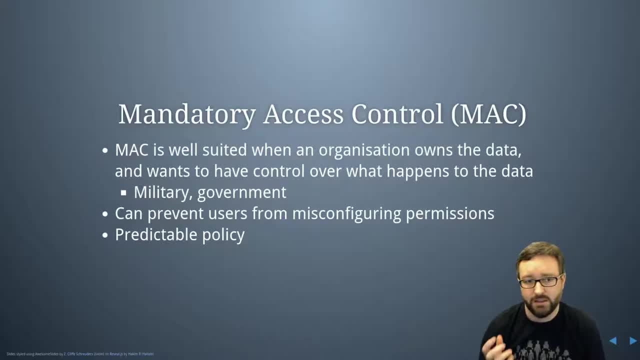 so, for example, the military or the government, um, so particularly military. so, um, you know, the nsa actually created se linux, um to basically introduce mandatory access controls into linux. but it can help to prevent users from misconfiguring permissions, because it takes all those powers away from the users, essentially, and it creates some predictable policy. 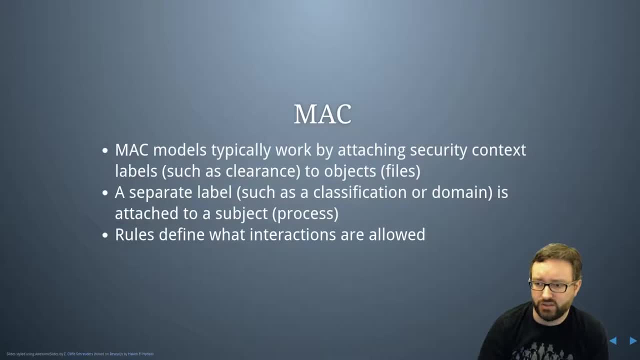 and some manager access controls. typically they work by attaching a security context label, like a clearance label, to the objects on the system and they attach a separate label, like classification or domain, to all the subjects or the processors and then you have rules that define what interactions are allowed between uh classification levels and clearance levels. 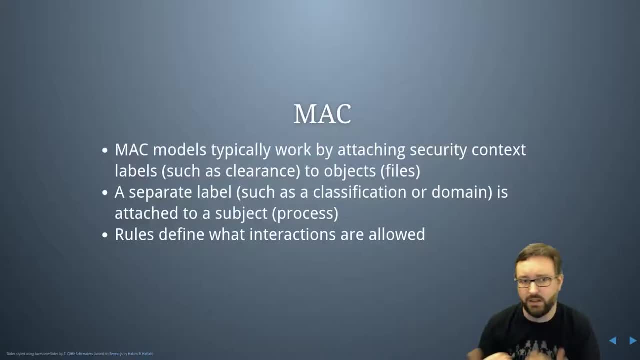 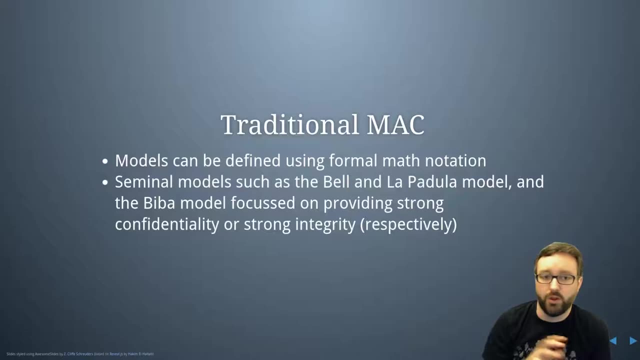 uh, so it's like you know. basically they have to match in order to access the file, for example. um. so, as i was saying before, traditionally the the models, access control models are defined using a formal math notation and seminal models like the bell and lapadula model or the biver model. 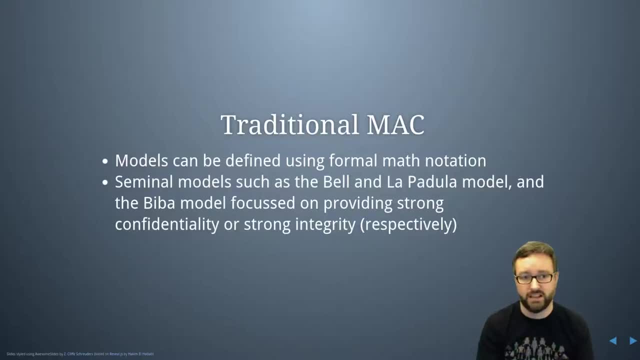 they're forced on providing either the strong confidentiality or strong integrity like separately. basically, in reality even the military want some control over integrity, even if is actually the highest priority. so in reality, you know, those models might not actually be used that much, because actually we need a hybrid of those kind. 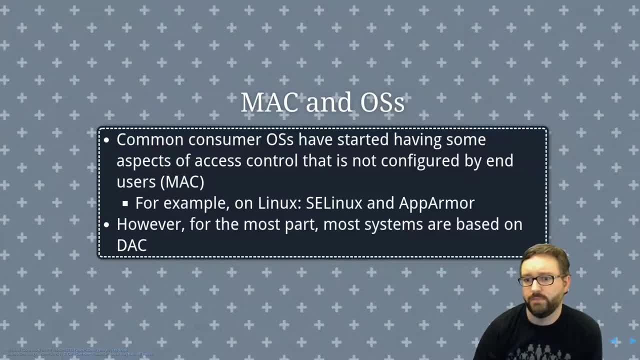 of objectives, security objectives. so now a lot of consumer operating systems have started to have aspects of access controls that aren't configured by end users, so it's a form of non-discretionary and mandatory access controls. so, for example, on Linux you've now got SELinux, which is was created by 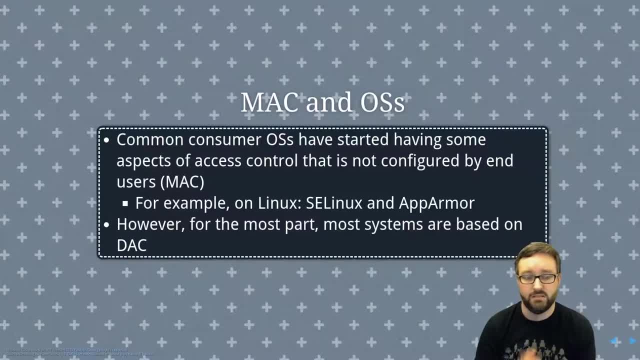 NSA, but it is. you know. you can use that to use like classification levels and to do multi-level security and domain and type enforcement and role-based access controls. it's just like mix of security models, basically, that you can define very, very powerful set of mandatory access controls. 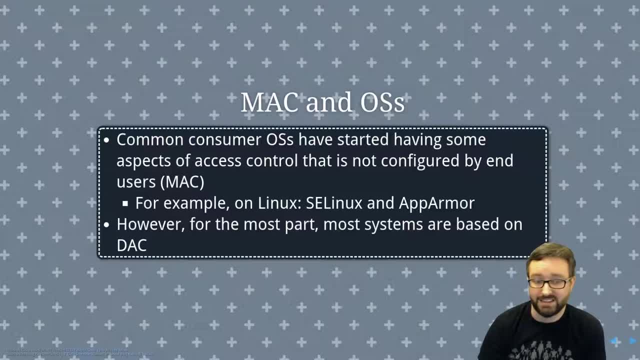 it's quite a lot of fun and it's a lot of fun to use and it's a lot of fun to use and it's quite complicated. the policy and and administering SELinux is is you know it's it's complicated but it's very powerful. AppArmor is a. 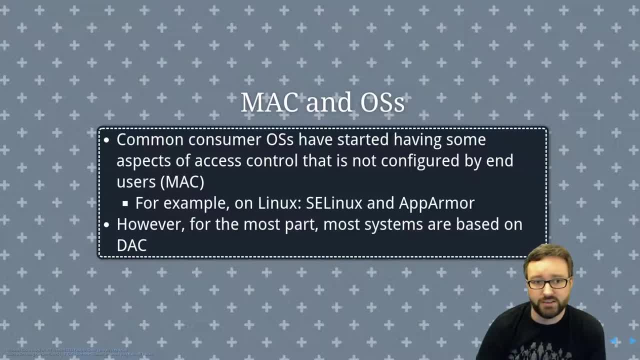 simpler managed access control system, which is a simple set of rules, but both of those systems control on a system level what different programs are allowed to do. typically, what you'll see is that you'll have administrators will use those systems to lock down. so you'll see that you'll have administrators who 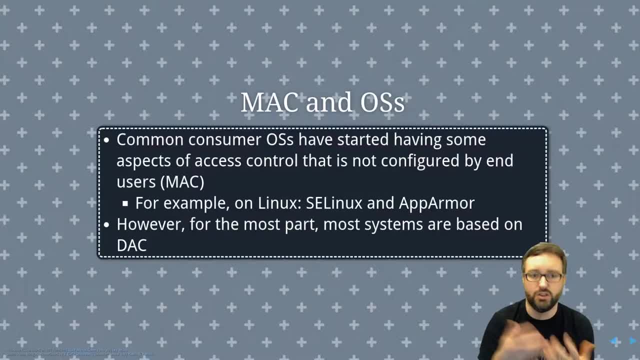 lock down services on a system and then you know users still get to use their discretionary access controls to choose what they do with their files. but then there's like the we'll use these mandatory access controls to add an extra layer of security. but yeah, for the most part, most systems are based on discretionary access. 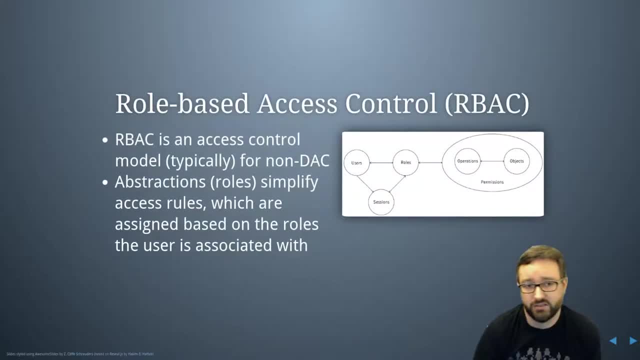 controls. role-based access controls is a. it's a way of using abstractions to set. it's typically it's non-discretionary, so you know the users don't get to choose. but the important thing is it adds this idea of a role and you have user sessions they get. 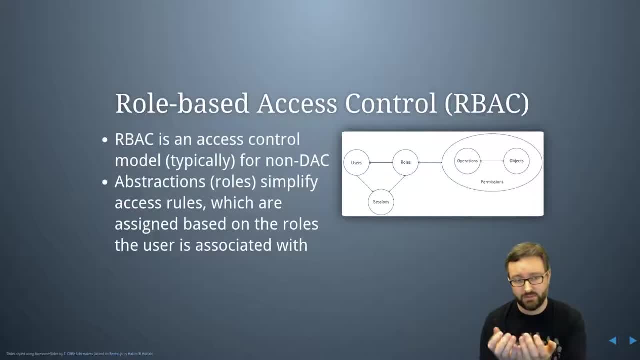 to use these roles. often they can activate or deactivate specific roles, which are often like hierarchical, so you've got a role that might be based on another role and it and it gives the users that have those roles a certain set of permissions. and so, for example, when you're 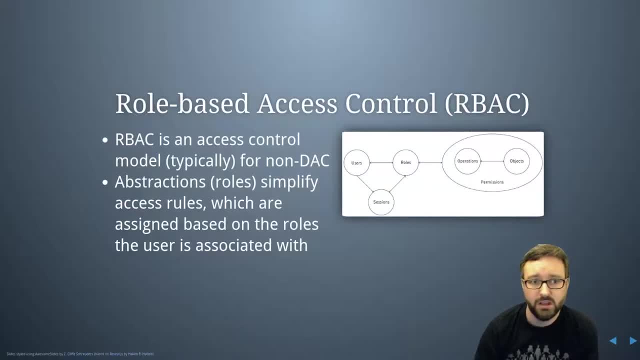 administering um, like the security for a hospital and you've got all the nurse in an organization. need nurses need to have a specific um set of privilege level. then every time you get a new nurse you just add: give them that role. but they might also be a nurse, but also a specialized. 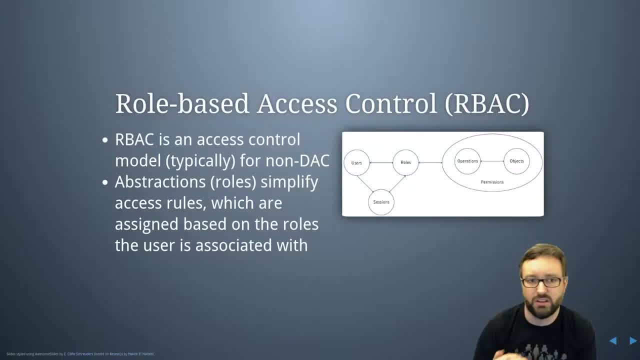 nurse or or a um specific doctor under certain um, you know, under certain conditions, and then they might also get those roles and that will give them access to those things as well. so it's similar to the simpler idea of using groups and access controls, but has extra features. 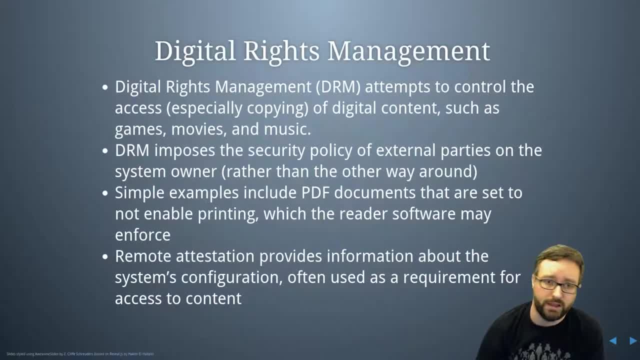 um, digital rights management is also a kind of access controls, although it's a little bit backwards in what it's intended for. so the idea of DRM is that you have these third parties that are providing some content and they get to choose how you use that content, and so they're trying to 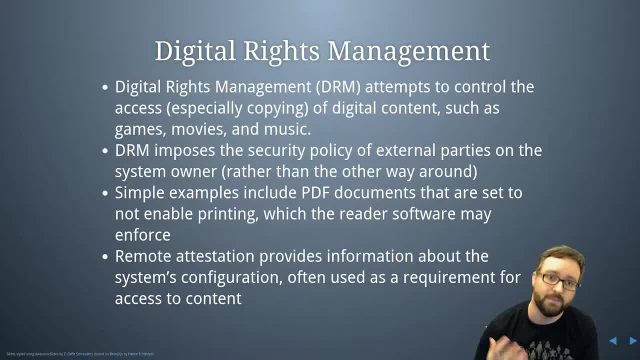 actually get you to enforce policy in your local machine, um, and so they define what the policy is on their systems and and you run get access to the media through software that doesn't let you copy it, for example. um, so the simple example, that is like a PDF document that has a some metadata attached to it that says, uh, 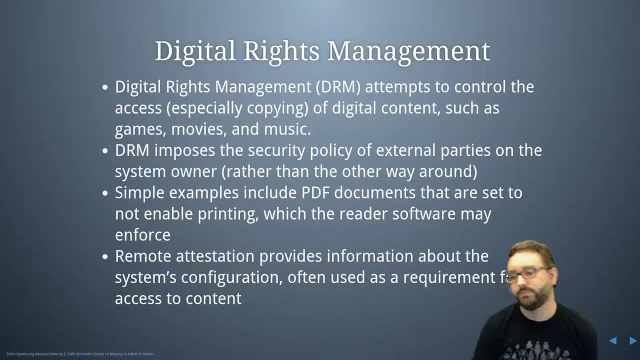 just, by the way, don't let the users print this file. now, if the software is behaving like you use the Adobe reader and it enforces that rule, then it won't let you print that file. um, however, you probably just download a different PDF reader and it will still let you print that file. so obviously it's quite easy to circumvent. um, you know that. 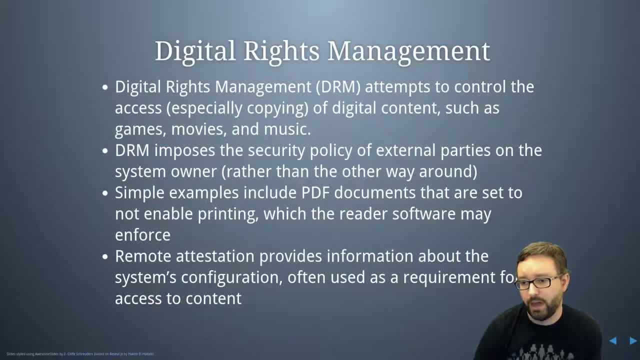 specific rule, um, but you know, unless they've got some even more complicated like um uh, encoding and encryption in place, that will only let uh authorized readers access the file, which is obviously what they try and do. um, you know, still, then you can take a screenshot of your screen so you know. digital rights management. 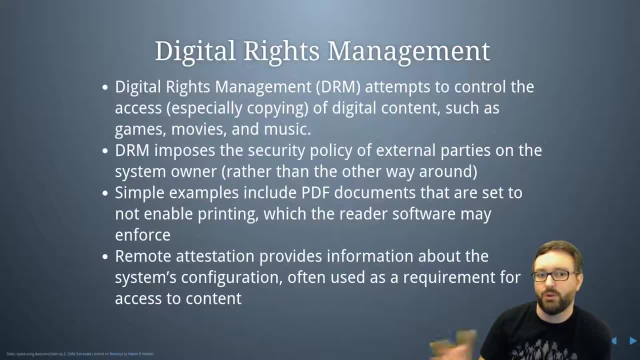 is quite obviously challenging, but they want to limit what you can do with the files and the resources that you have access to, and there's something called remote attestation, which is essentially where you prove over the network that the software that you've got running on your 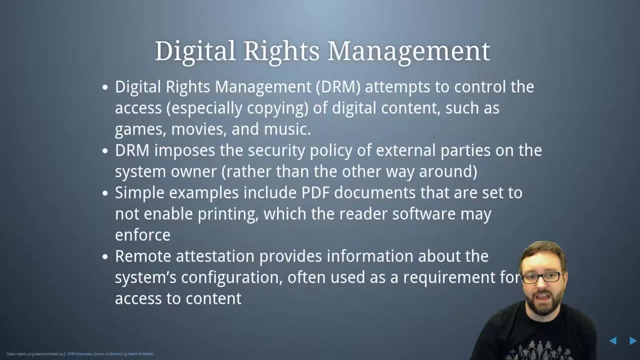 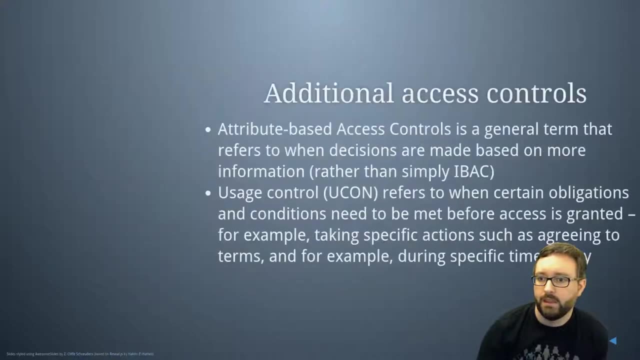 computer is limiting your actions, um, and and enforcing the DRM and then so it will check that over the network before it sends you a copy of your file, So that you know you then use that DRM software to access the files and just final, um, some more kind of terminology around access controls or some more kinds of.